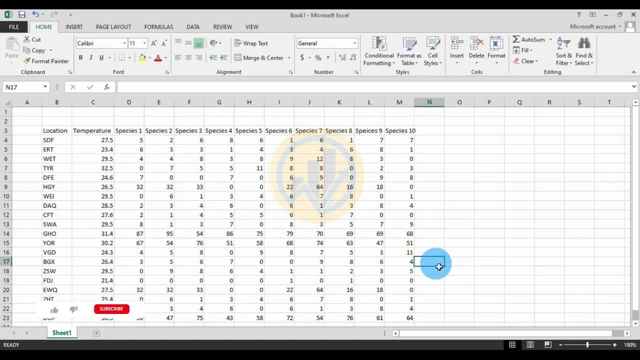 Hi everyone, welcome to statistics bios on youtube channel. Today we will discuss topic how to analyze it in the factor analysis with environmental variable. for the past statistical software, The data already entered in the excel sheet: The first one column for the locations, the 15 location. we take the different locations and the first one for the environmental. 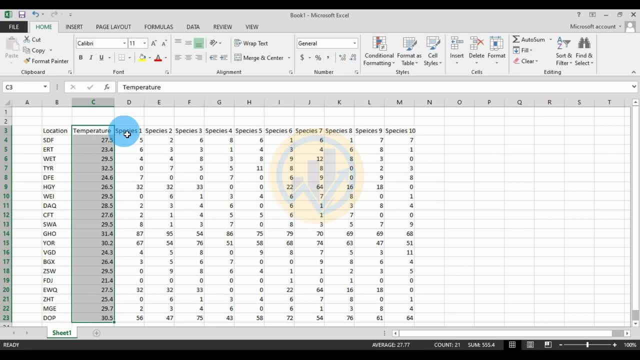 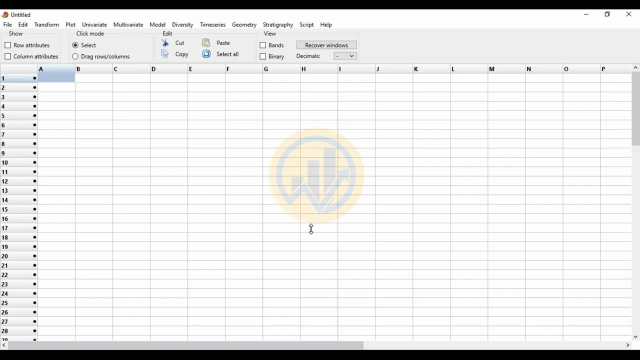 variable in the temperature. for measuring the 15 locations and the 10 species. for the 15 locations: distributions, the. now the copy, the data, the whole, the data. okay, hold the data selected under copy. go to the pass statistical software. then first click for the column attributed. 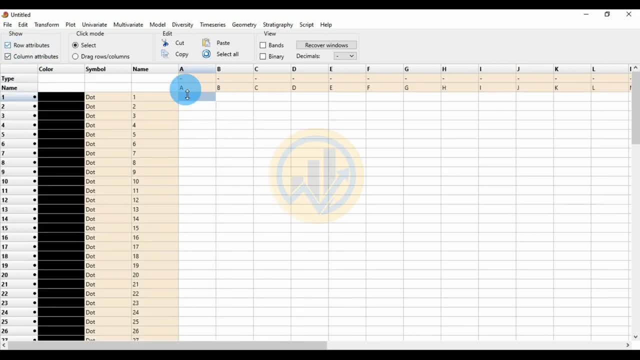 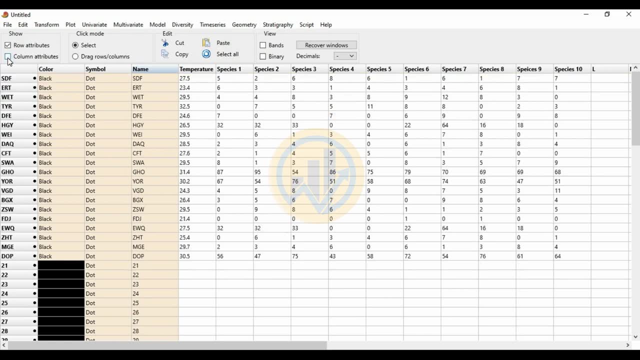 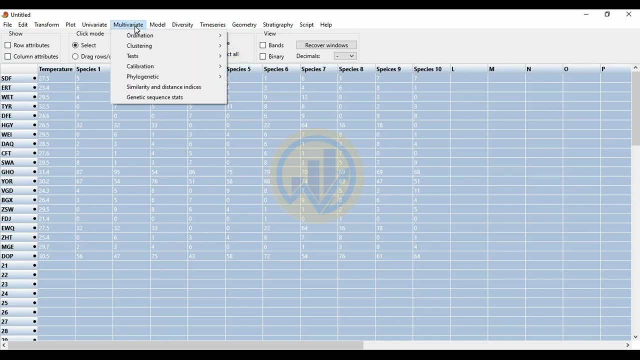 checkbox. under the row attributed checkbox. then select for the name, name, column, the paste the data. okay, then unclick for the column attributed checkbox and row attributed checkbox. then select the whole. the data go to the multivariate rated menu and the first one for the ordination and the click for the factor analysis: c a, b, f a c. 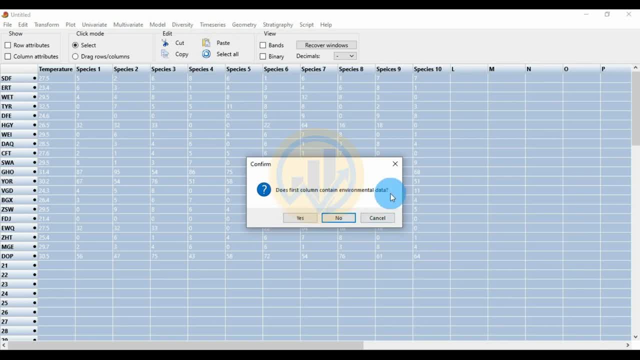 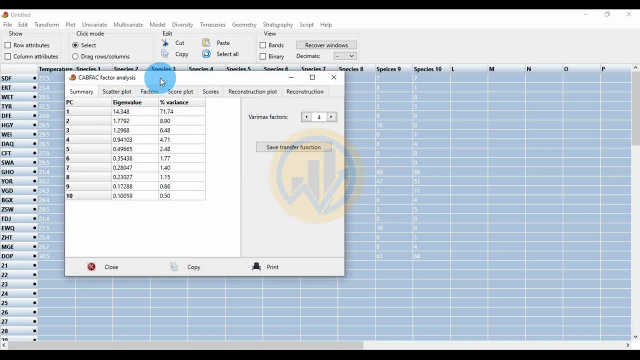 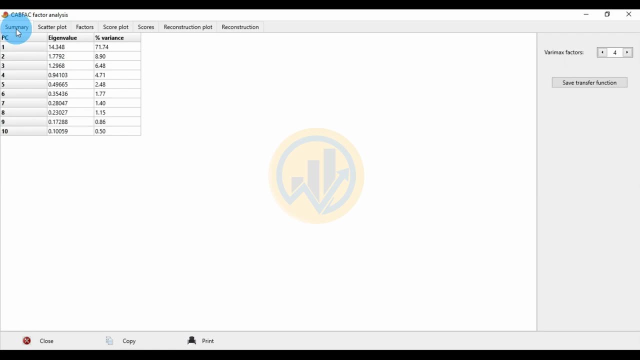 click it. if you do, first column contain the environmental data. yeah, the first column for environmental data and the temperature. so select the s button. okay, select the s button. open the new tab for the factor analysis with the environmental variable. the first one for the summary tab. summary for the 10 species. pc for the 10 species. 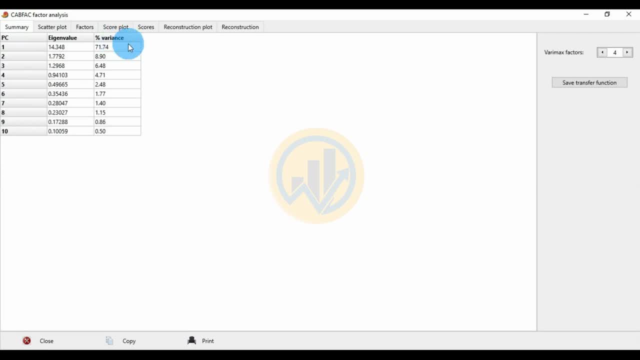 and the y n value under the percentage of variations. the maximum factor, the four factors then: pc, one for the highest eigenvalue, for the 14.348, and highest percentage, 71.74, and the lowest for the pc, for the 0,159. and the percentage of variation in the lowest, in the 0.50. 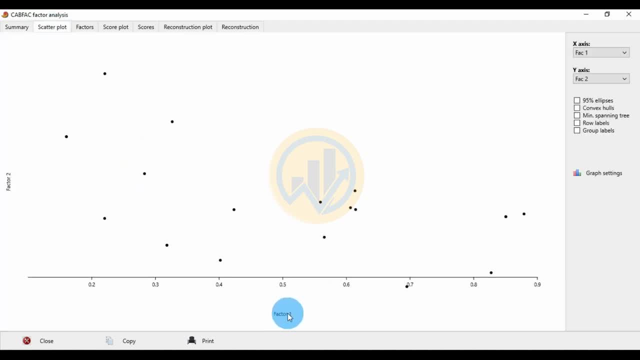 then next run tab for the scatter plot. this is a scatter plot for the factor 1 and factor 2 for the factor analysis with the norm delay variable. the factor anlamizer is, with the non-delay variable, the first cell for the XS in the factor one, the YHS is a factor two, if you change. 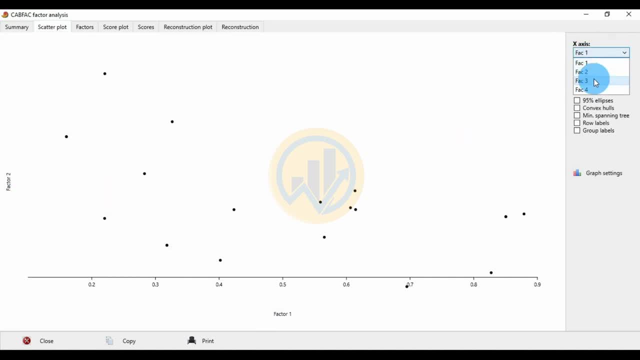 the factor, the four factors: the XS for the factor one or two, comparison to the X factor two and the XS factor three, comparison for the XS factor two. and if I XS change to the factor four and the YHS factor two, then a standard selection for the factor one to factor two for the XS and YHS. the first one checkbox, the 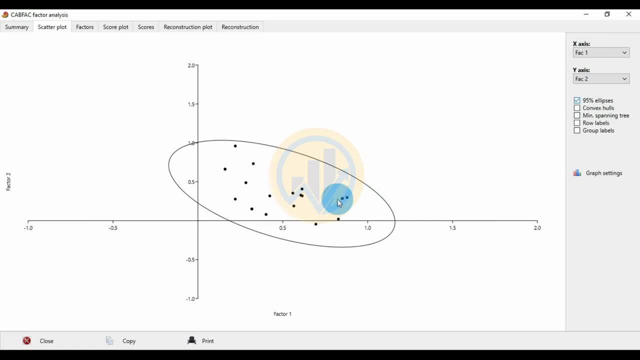 95% epsilon, the rounds and all the species are covered in the location for the 95.0 EPSILONs. then next one for the convex scales, the connected to the outer side location for the species. the next one, minimum spacing tree, the connected for the tree for the species distributions. our next, 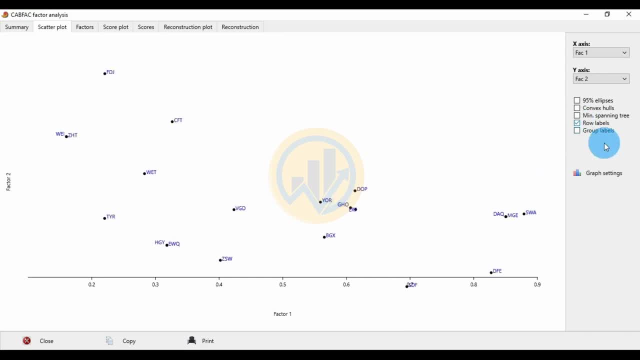 one for the checkbox, the row label, the row labels. select the all, the location and names. then next one for the all, the group label. this is a factor one and a factor two and the factor three for all the group labels, then next one for the factor 2, the next one for the scatter blood score, for the factor 1, factor 2, factor 3. 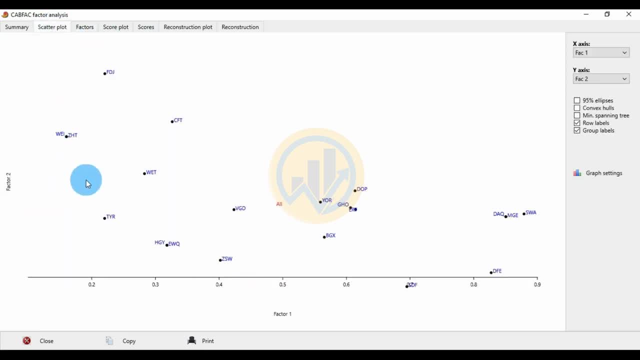 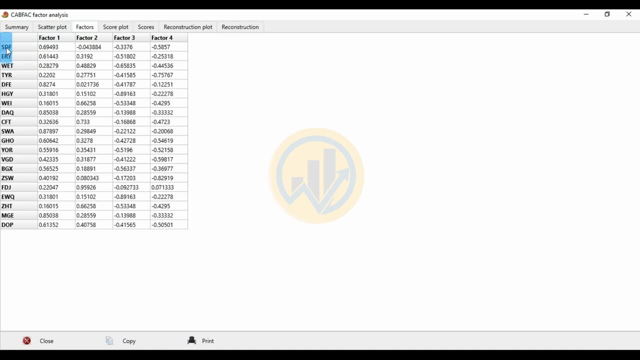 and the factor 4, this is factor 1, this is a factor 2, now this is 95% epsilon. this is cover for the factor 1, the factor 2, the range of the factors, the SDF, the positive. 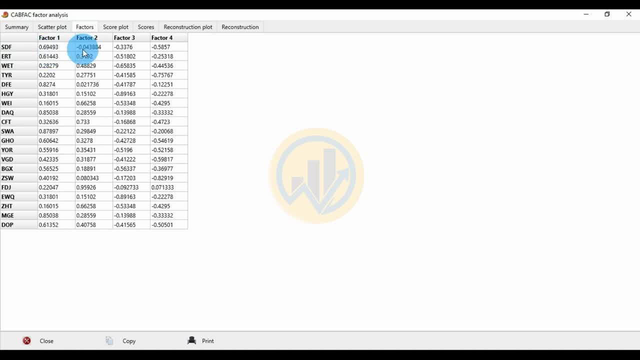 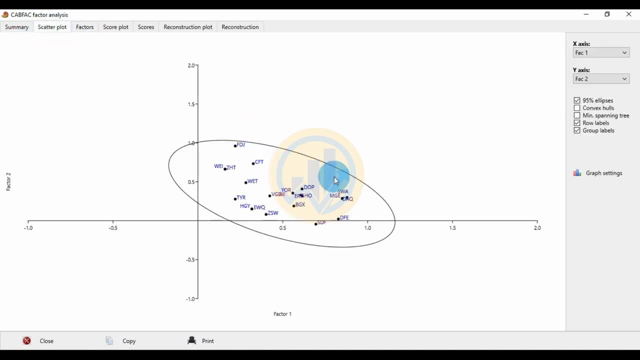 for the 0.69493 and factor 2, minus 0.04384, SDF. where is the present of the SDB? this is a SDB: the factor 1 presented in the positive value, at same time the negative for the factor. 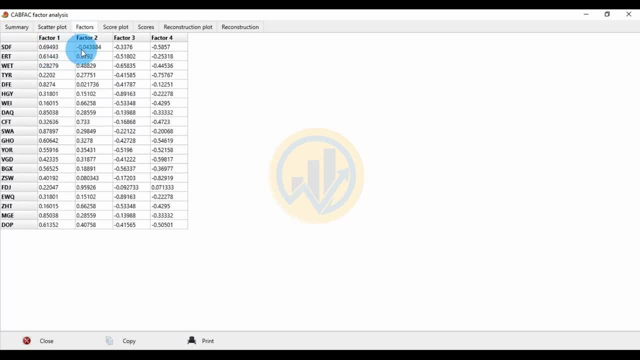 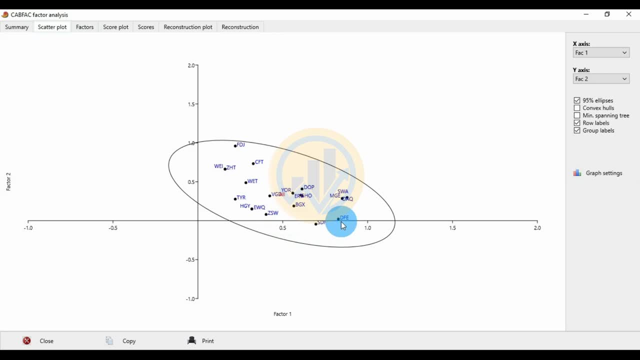 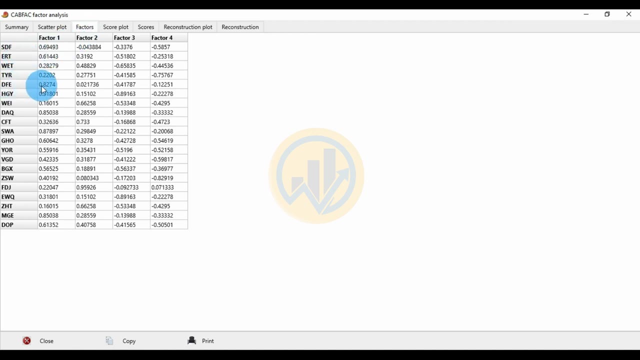 2, the positive value for 0.69 and negative for the 0.04,. this is a 0.04 and 0.09, the next one for the upper upper right column, for the DFE: the value for the DF value. DFE: the positive for the. 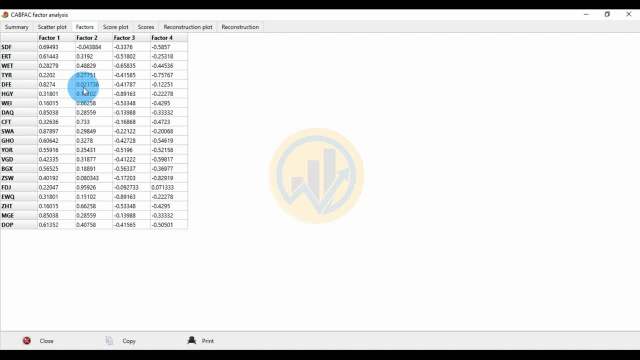 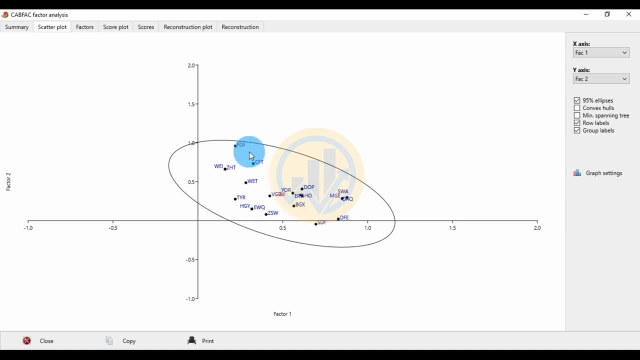 0.82 and at the same time, the positive for the factor 2, 0.02,, 0.82 for the factor 1, the factor 2, 0.02, this is a scatter blood for, with the nominal variable, the factor. 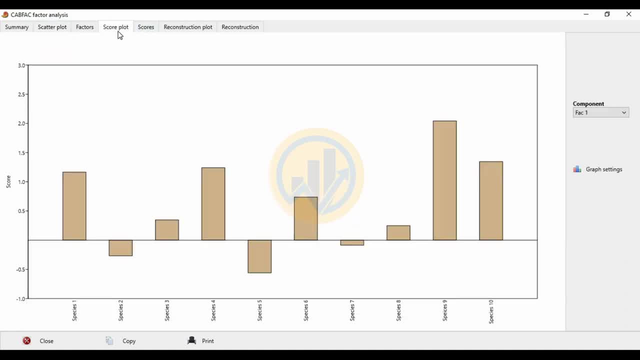 analysis in past statistical software. the next one for the scatter blood, the score blood for the 10th species in the factor 1, 4, 2, 3, 4.. This is a factor 1 for the only 3 species in the negative value presented. the next: 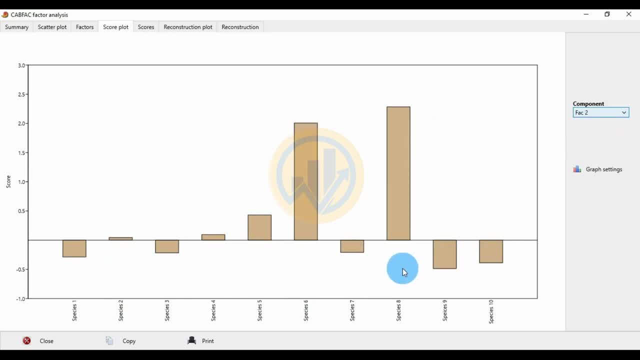 one for the factor 2, the 4, 5 species present in the negative value, and the factor 3, is a 1,, 3,, 3,, 6,, 7 species presented in the negative value, the highest present in the species 7.. 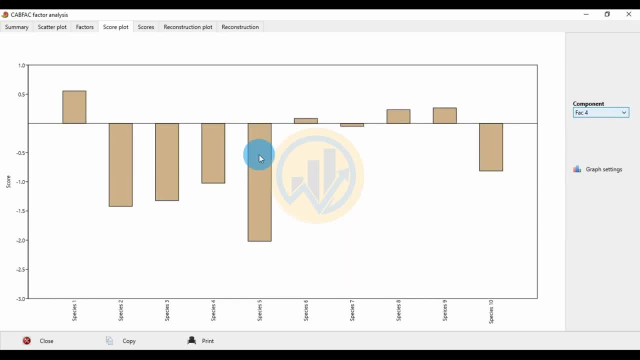 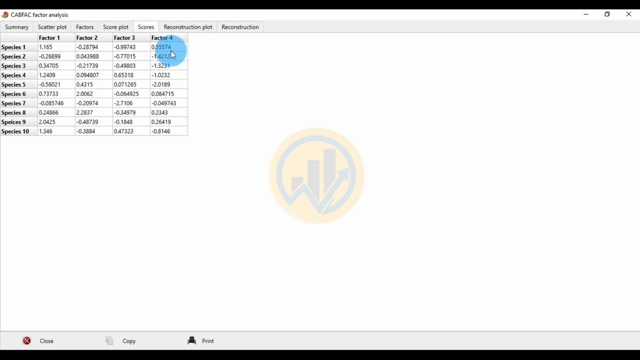 Then the factor 4, the comparison for the same the 6 species presented in the negative value then go to the for the score for the. this is factor value for the factor 4, the score for the factor 4, the species 1, 0.55574,. the species 1, 0.4545,. this is the score value. 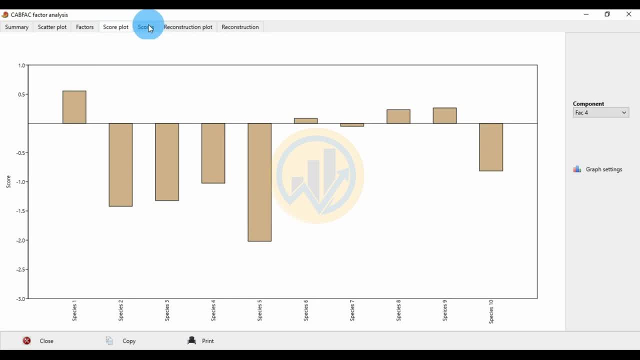 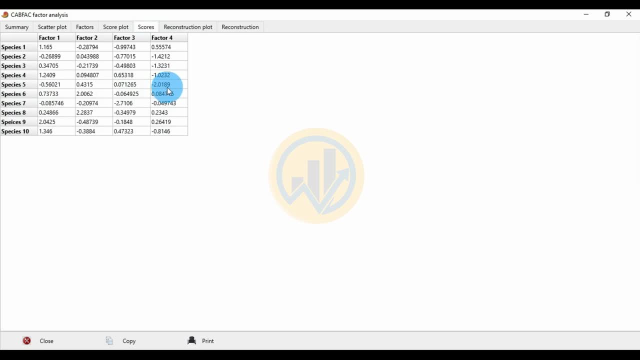 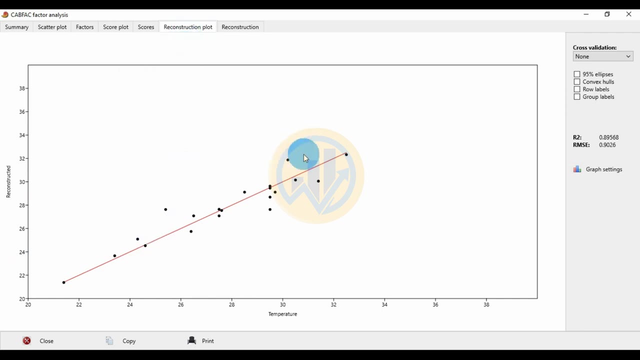 the next one highest: the species negative value present in the species 5,. this is a species 5,. the highest negative value for the minus: 2.0189,. the next one for the reconstruction plot. This is for the important for the, with the environmental data only available for this. 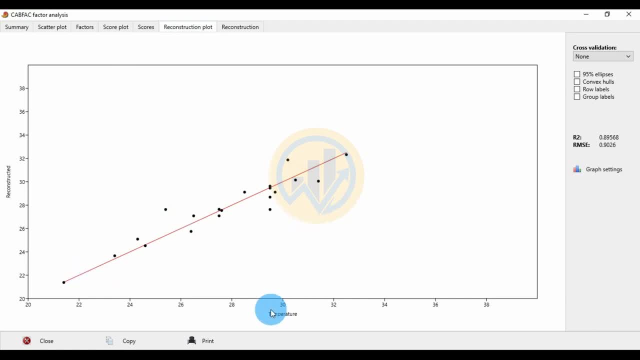 plot for the reconstruction plot. This is a temperature, the xs for the temperature, yk for the present and the reconstructed. This is a crossing validations. the level of 1 out, okay. the next one for the 10 float, then 5 fold, then 2 fold- okay. the standard for the none. 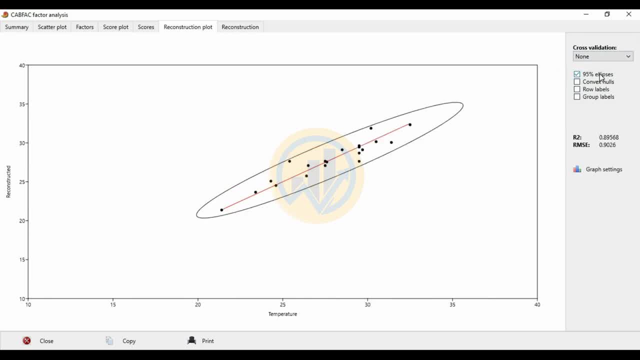 Okay, again, you can put the 4x3 episode cover that. So click the check box, all the site locations, then Then next one for the low law row label for the species distribution locations, then on the group label, then R-square value for the 0.8564. this is a positive correlation. 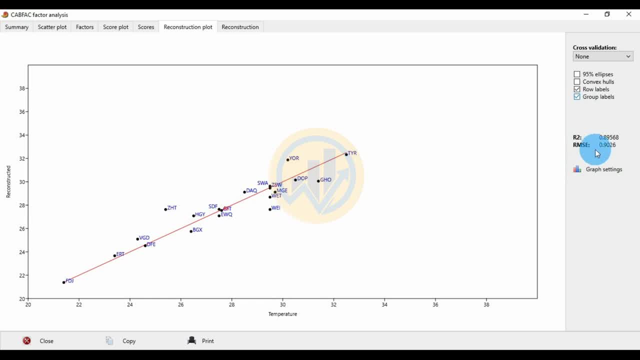 value and the next one for the RMSE value for 0.00 foram. stretch value for the 0.9026.. This is also the positive correlation value value for the r square value and rms e value also. okay, then next part of the reconstruction. 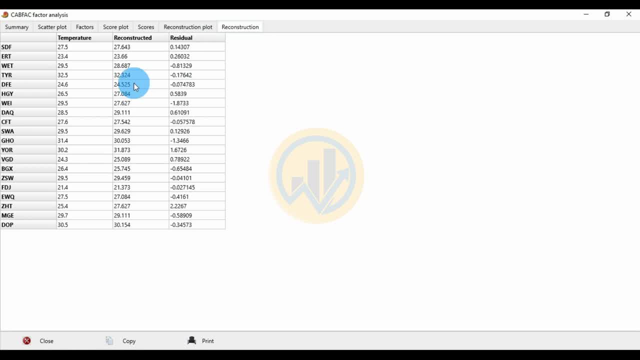 the plot value presented in the next one tab. this is a reconstruction plot value. this is a temperature for the 15 location site, the highest presented. the temperature for the gh locations then, 31.4 is the highest percentage of the temperature. the species distribution also the 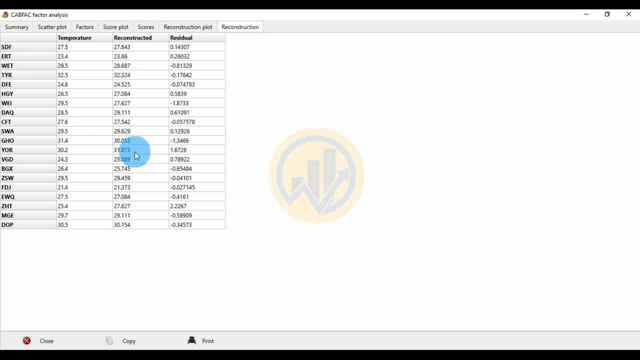 reconstructed: the highest and the 31 point for the 873 and the lowest for the 1.627. this is a construction rest cell. okay, this is for the data for the temperature and reconstruction, for the reconstruction plotted. this is a plot for the reconstruction plot. this export for the plot how. 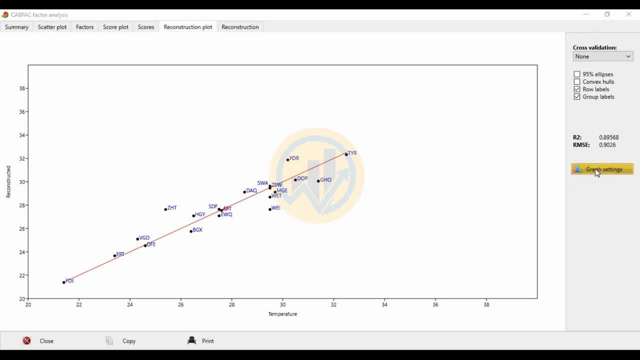 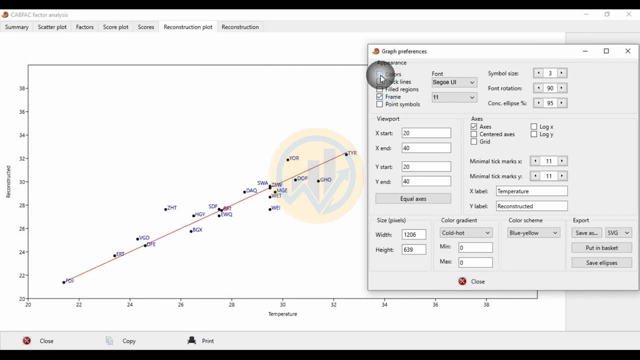 to the export plot. this is a setting for the crop setting. okay, click the crop setting. the open the new tab for the crop. reference the person for the color. this is a color. if you want the color or non-color, this is the color. this is a grass scale. then pick layer, then okay, then increase the symbol size of. 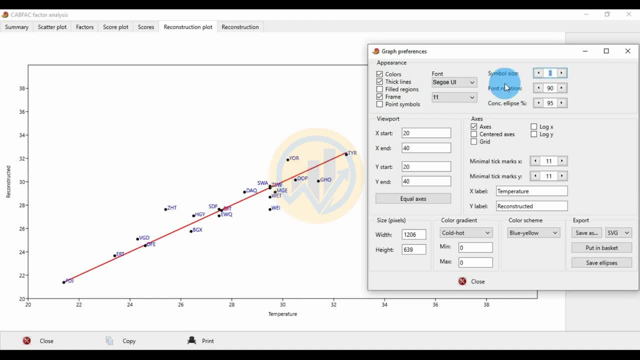 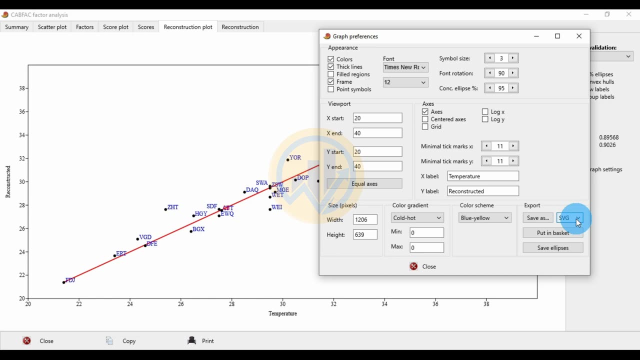 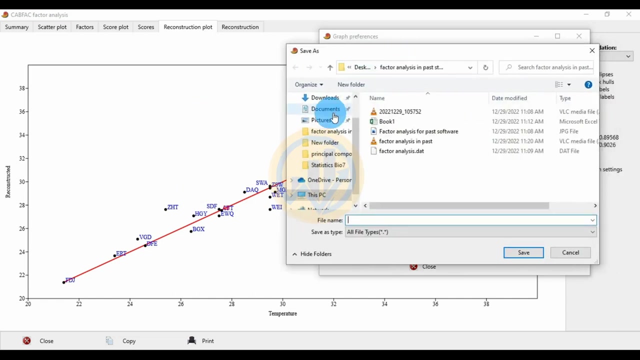 four, five, six. okay, the standard three. okay the change the font. set the time. roman font size: 12. okay, this is a format for the export to the jpg format. just click the save as button. okay, then factor in normal with the normal the save. enter the name: reconstruction plot. 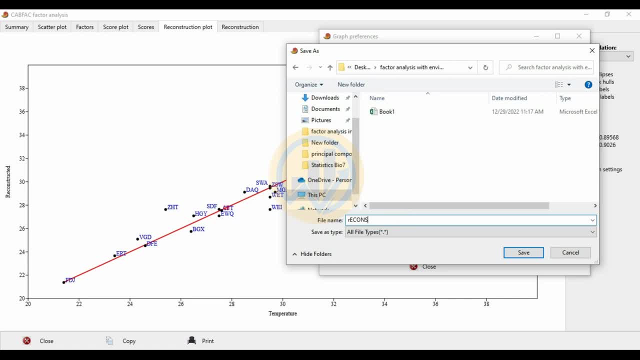 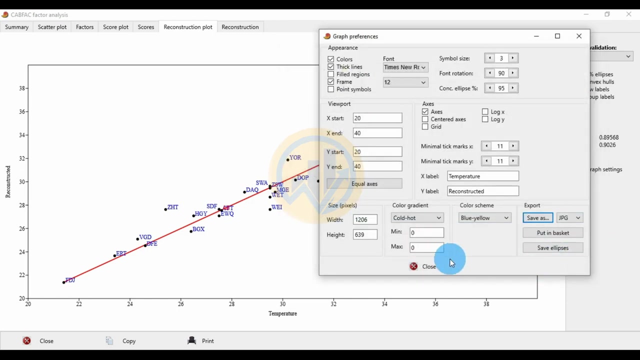 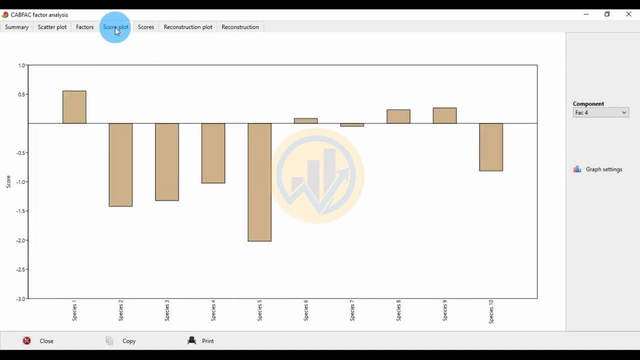 reconstruction plot. so nao tree isato, no fees. Okay, save it. This is one of the graph. are the reconstruction pattern in the factor analysis, Then the next. the next one graph for the score plot. this is a change for the factor one, then next one plot for: 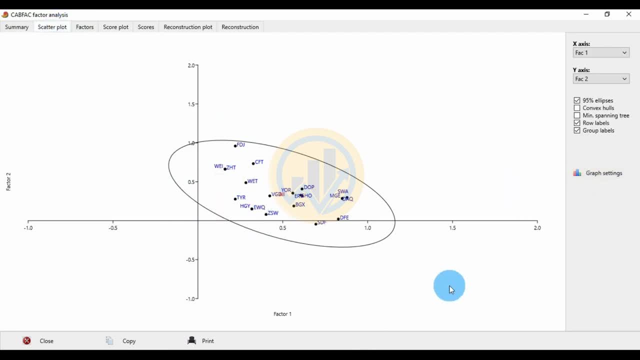 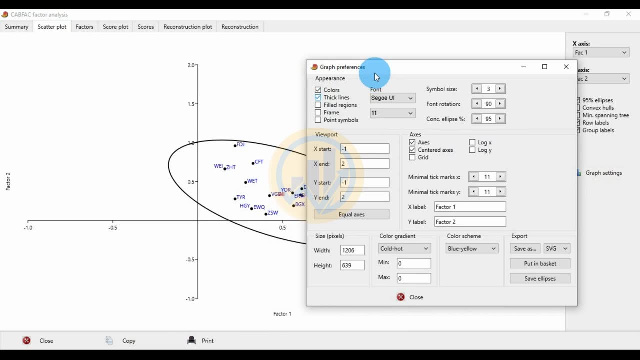 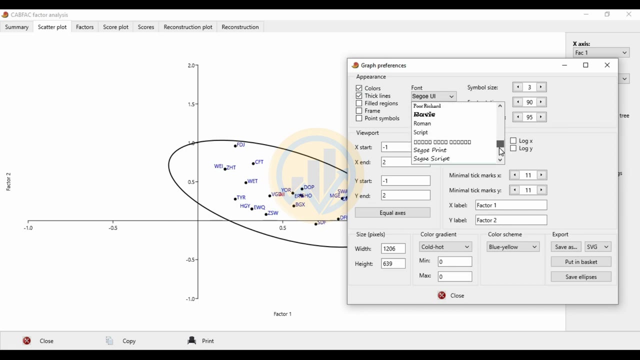 the scatter plot. this is a save to scatter plot. for the go to the crop setting. click the crop setting. the same, the setting for the thick layer, thin line and the change for the font, the time Roman font size for the 12. okay, they save the format for JPG. save as button. click the export.